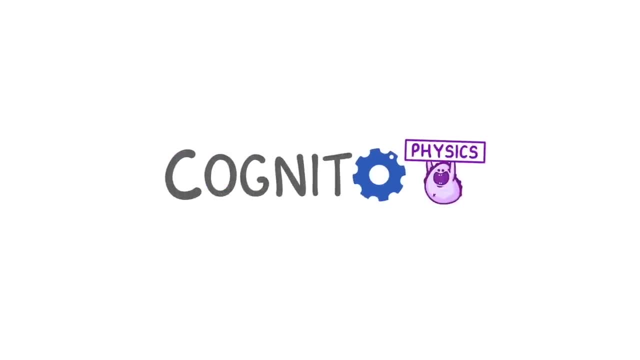 Today we're going to take a quick look at orbits. We can describe an orbit as the curved path of one celestial object or spacecraft around another celestial object. So this could be the Earth orbiting the Sun or the Moon orbiting the Earth. The question we're going 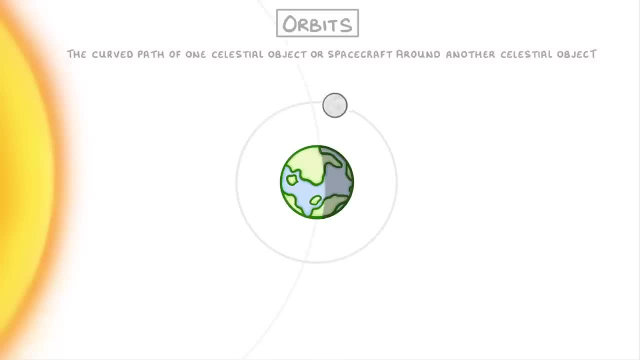 to try and answer during this video is to explain why objects actually orbit like this, rather than just flying off in a straight line or being pulled in towards the object that they're spinning around. Well, we know from Newton's first law that an object travelling at a certain velocity 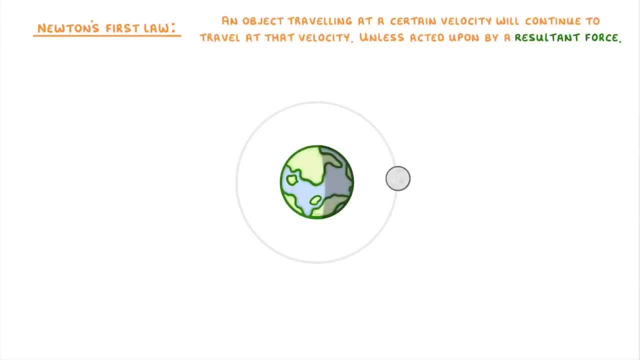 will continue to travel at that velocity unless it's acted upon by a resultant force. So if the Moon is travelling at a certain velocity, it will continue to travel at that velocity unless it's acted upon by a resultant force. So if the Moon is travelling at a certain velocity, 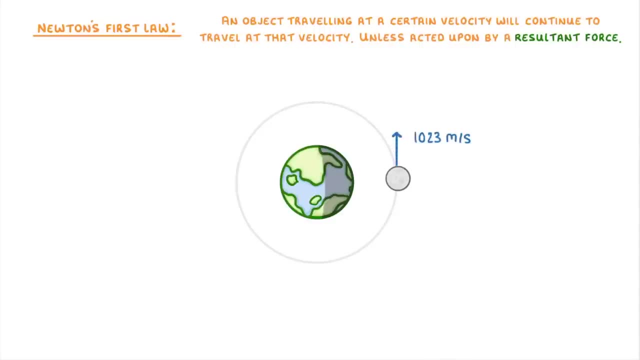 if the Moon is travelling in this direction at 1023 metres per second, which we call its instantaneous velocity, then it should continue to travel in this direction and at this speed forever. However, because the Earth is so massive and relatively close to the Moon, 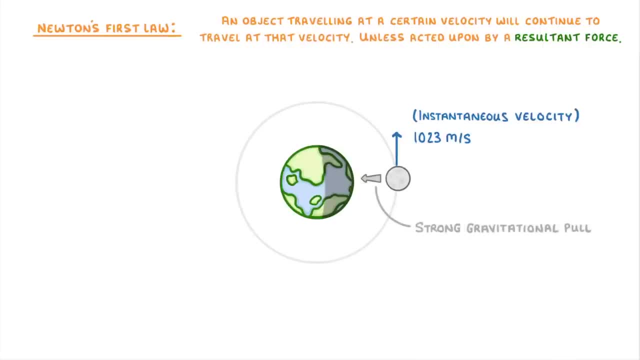 it exerts a strong gravitational pull which is felt as an attractive force towards the Earth. Because the Moon is quite big and travelling very fast, it has a lot of momentum in this forward direction, And so the gravitational force isn't strong enough to completely pull it in towards the Earth. It can only change. 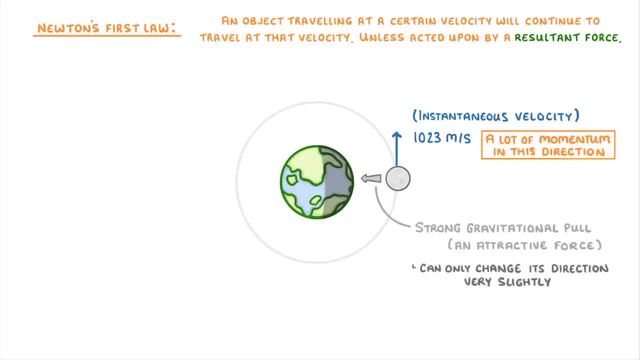 its direction very slightly, As the Earth is always applying this gravitational force, though it's always changing the Moon's direction. So in practice, this means that the Moon is basically always orbiting around the Earth. Now, one of the confusing things about this situation is that, even though the speed of 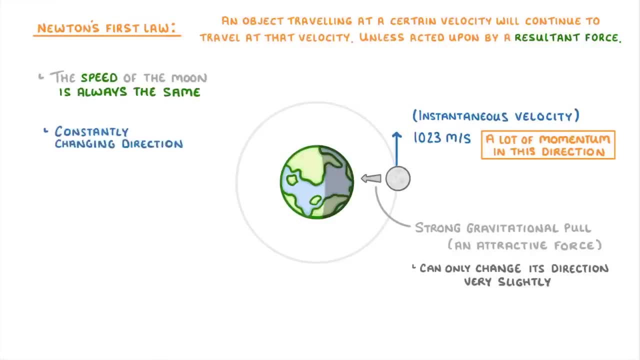 the Moon is always the same. it's constantly changing direction And because velocity measures both speed and direction, this means its velocity is constantly changing. So if we remember the equation for acceleration, we can see that any change in velocity must mean an.